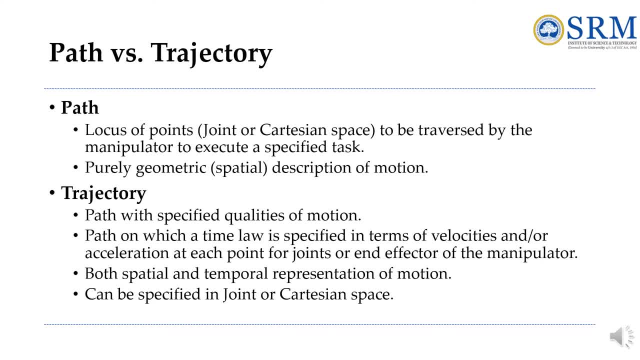 is, it is concerned about when each path of the path must be attained. Thus it specifies the timing, So path purely describes the geometric description of motion and the trajectory which represents, in both spatial and temporal representation of motion. So as the trajectory specifies the timing, so this can be specified in terms of velocities or acceleration at each point for joints of the manipulator. 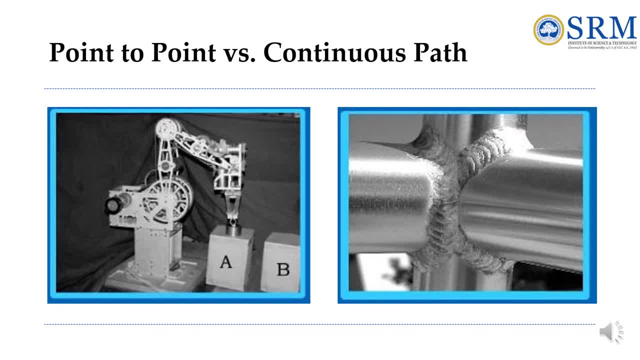 So next is the what is point-to-point motion and continuous path motion. So point-to-point motion, which teaches initial and final points, intermediate path is not critical and it is computed by the controller. So applications here included are moving of parts, spot welding, automated loading and unloading of machines, pick and place motion. all these comes under the point-to-point motion, trajectory planning and next is the continuous path motion. the second picture shows the continuous example for continuous path motion. 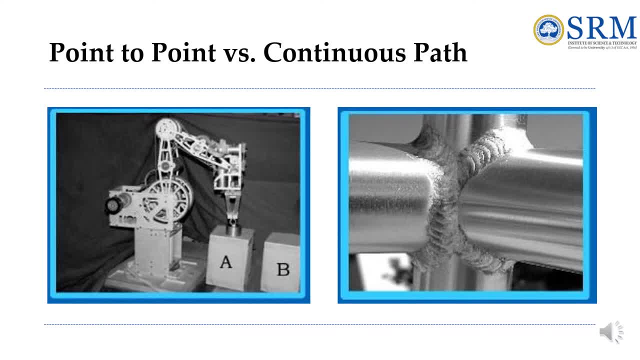 So this is used when there is a need to follow a complex path. Who 3d space? so possibly at high speeds. For example, you can think of a spray painting, welding, polishing, And this points generally taught by manually through with high speed automatic sampling. 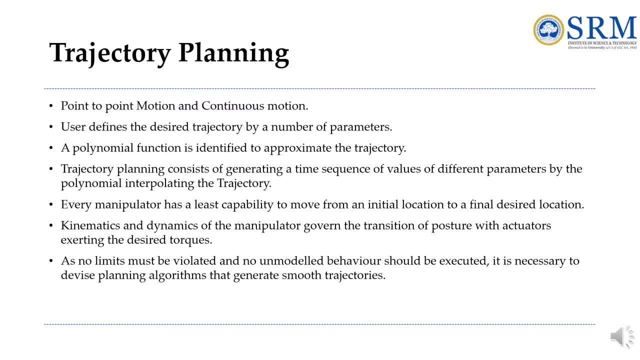 So first it checks whether the application is based on point-to-point motion path or continuous motion path, and the user defines the desired trajectory based on three priorities: ieelet, memory, ree, hated data and chip- by the number of parameters and a polynomial function is identified to approximate that. 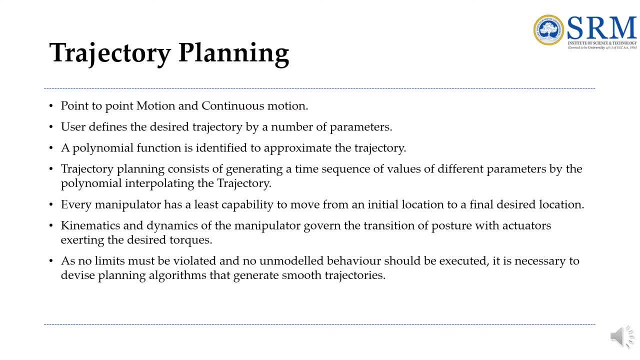 trajectory. so this trajectory planning, which consists of generating a time sequence of values of different parameters by the polynomial which interpolates the trajectory, and every manipulator has a least capability to move from an initial location to final desired location, that is, from one point to the another point: kinematics and dynamics of the manipulator which governs the 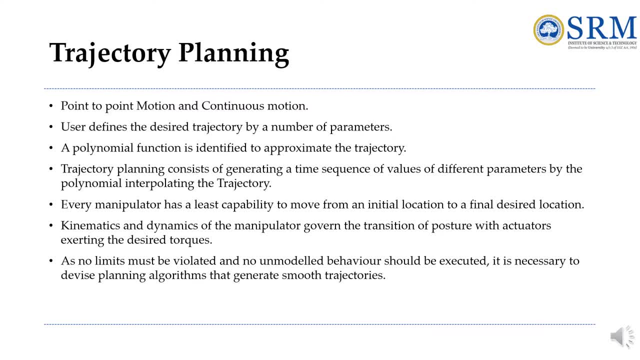 transition of posture with actuators exiting the desired tux. so whether it uses the inverse kinematics for finding the corresponding path for the joints in the joint space, or it used the inverse kinematics for finding the initial and final joint portion in the joint space, so it used both cartesian space techniques as well as the joint space techniques to compute it. 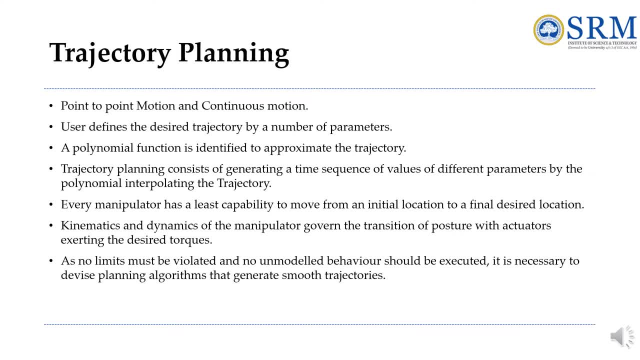 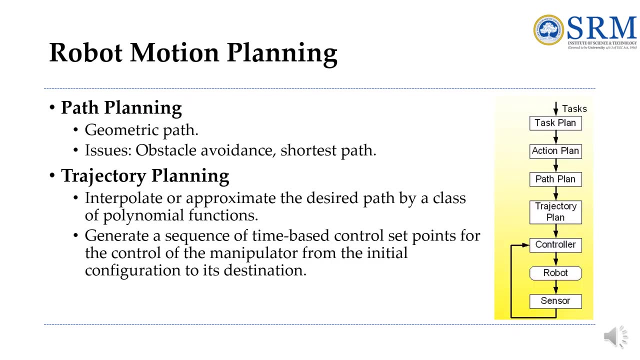 and as no limits must be violated and no unmodeled behavior should be executed, it is necessary to devise planning algorithms that generate this smooth trajectories. next is Robot Motion Planning. it could be a path planning or a trajectory planning. in path planning, it has path description, path constraints, that is, obstacles and this. 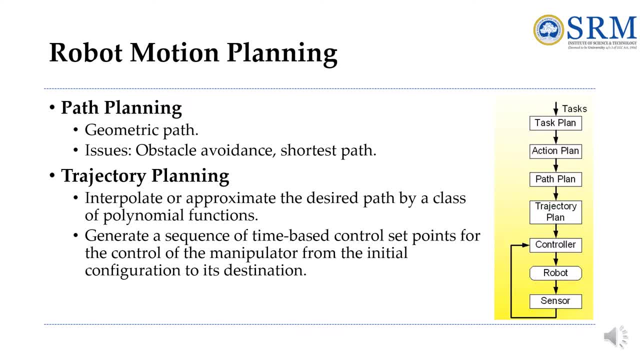 constraints are imposed by robot dynamics. and the second one is the trajectory planning, where joint trajectories in terms of position, velocity and acceleration is identified. in the first method, we plan a path in Cartesian space and it used inverse kinematics for finding the corresponding path for the joints in the joint space, and this uses the Cartesian space techniques and the 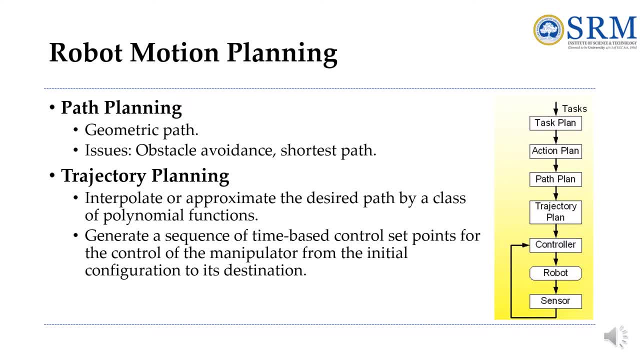 second method: it used the inverse kinematics for finding the initial and the final joint position in the joint space and plan a path in the joint space. since computing the inverse kinematics in real-time time consuming the " method one is time consuming and robot efficiency may be affected. so when this is used is when a 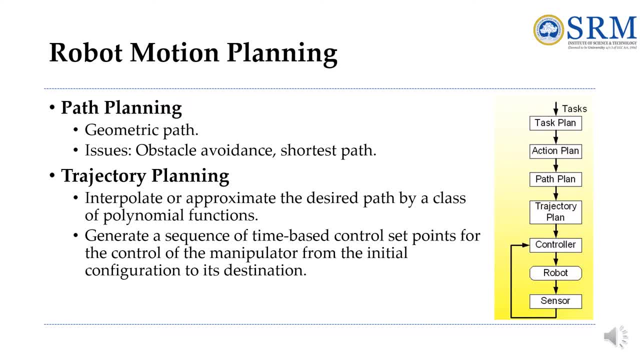 specific end effector trajectory is required. in that time this method is useful. example in say, in the case of arc welding, or the electrode is required to follow the seam precisely in that case method one is useful. and then second method: it determines the initial and final joint positions. 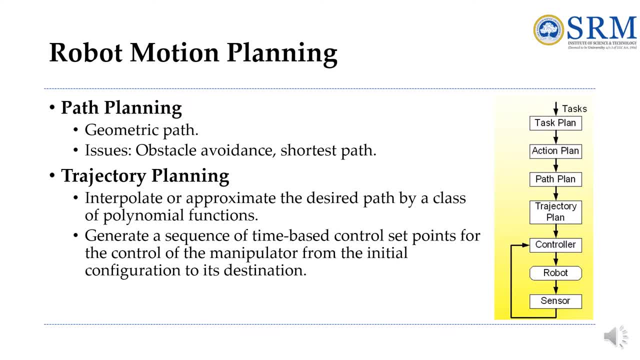 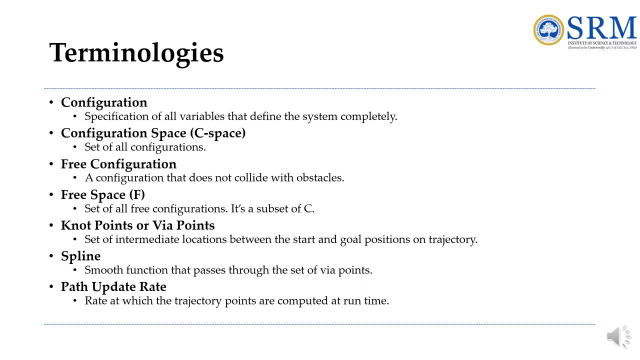 so the path for all joints can be easily planned in the real time. in this case there is no need for the forward and inverse kinematics recalculation. there are some of the terminologies which is used in trajectory planning are listed here first. one is configuration, so it's specification of 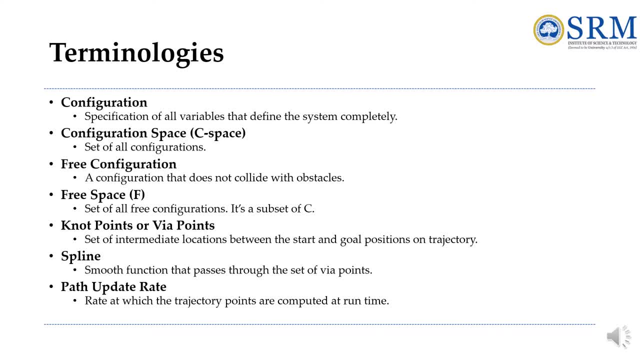 all variables. which defines a system completely is a configuration, and the configuration space is a set of all configurations, and free configuration is the one that does not collide with obstacles. and you have 3 space, which is denoted by F. it is a set of all three configurations and it's a subset of the configuration space. you 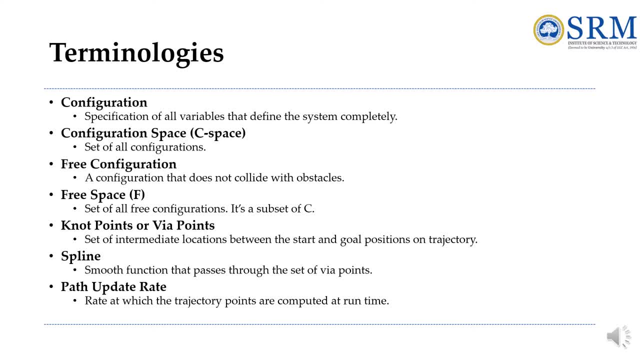 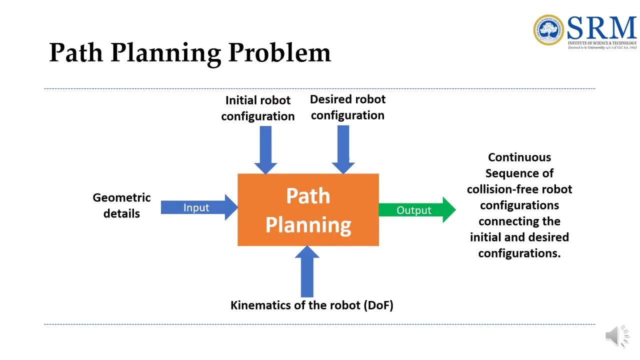 have not points set of intermediate locations between the start and goal positions on the trajectory and you have a spline, which is, which is the smooth function that passes through a set of not points, and path update rate. this is the rate at which the trajectory points are computed at runtime. next is the path planning problem. so here the problem statement could be: 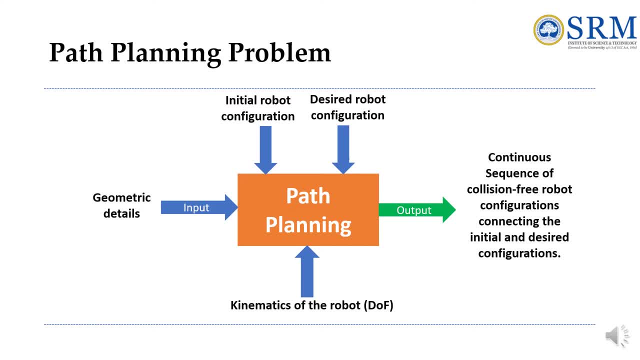 we have to compute a collision free path for a rigid or articulated moving object among the obstacles. and here the input is geometry of a moving object- here it is a robot or a molecule- and obstacles. then we have to see how does the robot move, so it is econometrics of the object robot, that is, degrees of freedom and also its position and 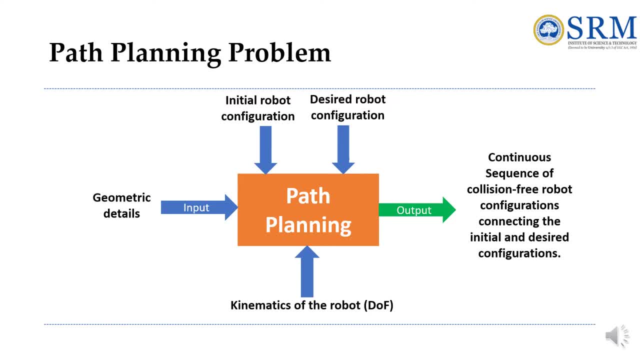 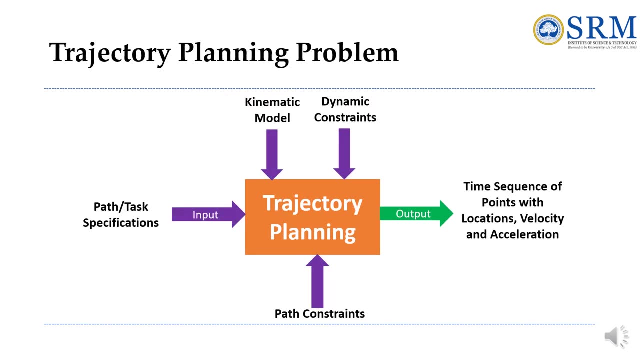 orientations, which will have its initial and goal robot configurations and obviously the output will be the continuous sequence of the collision free robot configurations which connects the initial and goal configuration. next is the trajectory planning problem. so the problem statement could be a specified cartesian space trajectory into a appropriate joint position reference values, and here the input is cartesian. 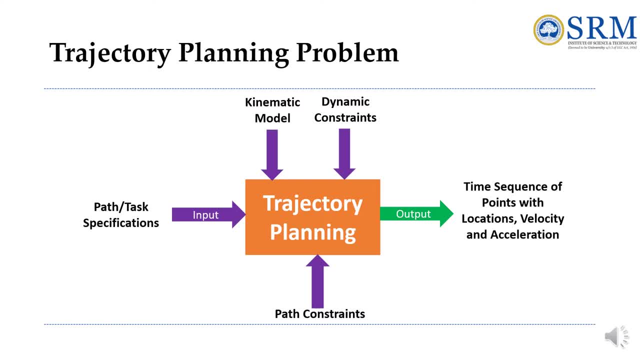 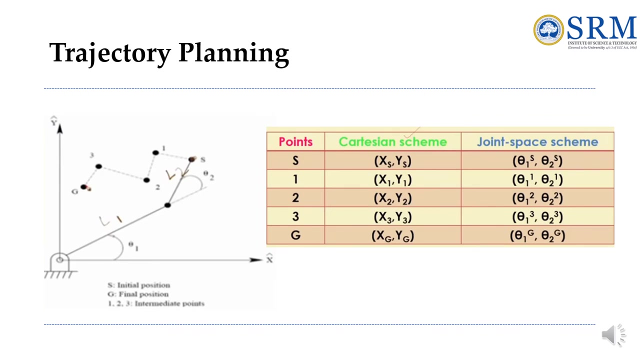 space path, so the path can. constraints, which includes velocity and acceleration limits, and also its singularity analysis. so the output here is the series of joint position or velocity which depends on this particular light and according to the input value we can calculate the knowing of the distance from the particular side. and on the surface, so we can calculate the 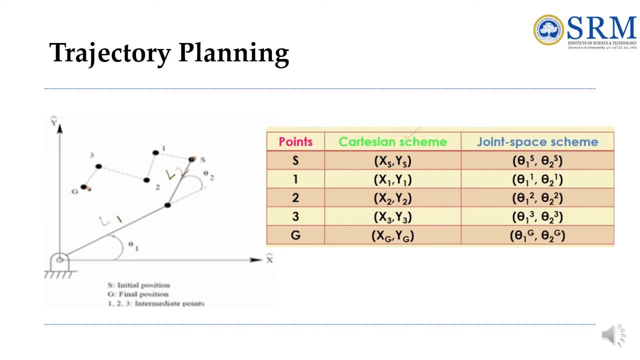 distance y is the distance between the object and the object is 1 by 3 and 2, and the distance between the object and the object is 2 by 2, so this gives us the three points, which is z, 6, 7, and the distance between two objects is 3.5 and so forth, and the distance between those objects is. 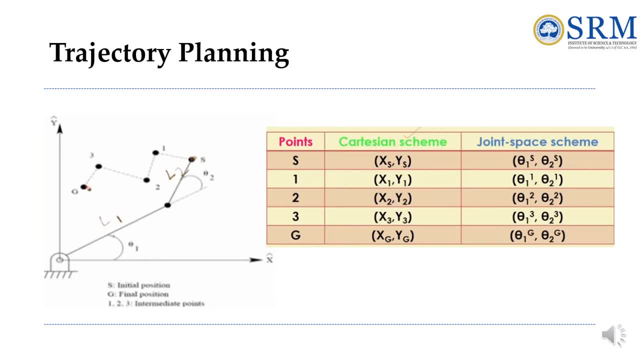 4.5. so this is the number of points which is equal to the velocity and acceleration limits. if the reference values are 0, the total variation of the position will be order t in general and the 402 values. So the output here is a series of joint position or velocity reference values to send to the 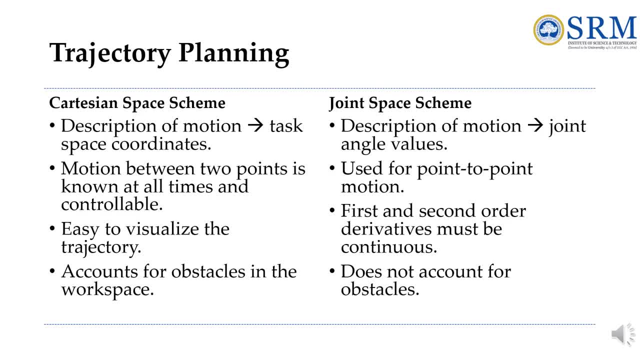 controller. So the trajectory planning is carried out both in Cartesian space and joint space. So Cartesian space, which uses the task space coordinates, that is, the Cartesian space coordinates, and joint space uses the joint angle values. Cartesian between two points is known at all times and it is controllable in case of 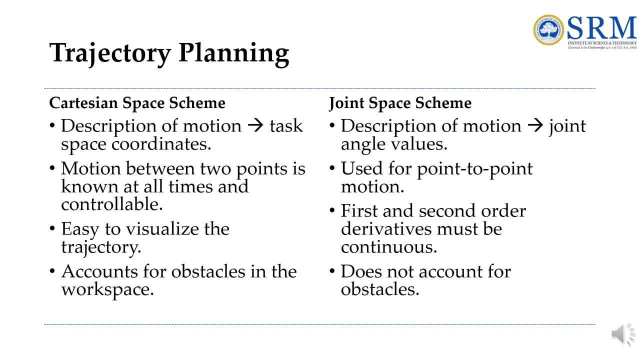 Cartesian space, and here this is used for point to point motion and in Cartesian it is easy to visualize the trajectory. and in joint space scheme first order and second order derivatives must be continuous. Where Cartesian space it considers the obstacles in the workspace And in joint space it does not account for the obstacles. 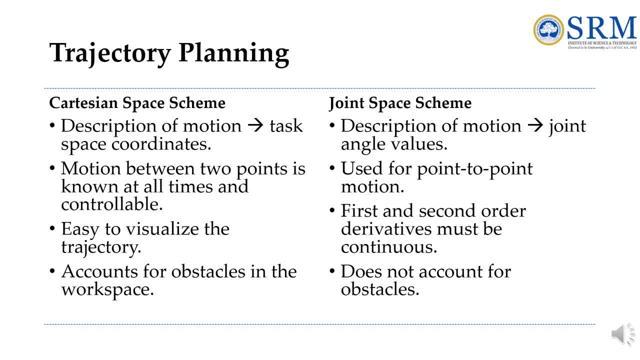 And in Cartesian space inverse kinematics problem has to be solved. computational complexity is there. it reduces trajectory sampling rate in real time operation and trajectory tracking accuracy decreases in this and there is a. there are problems with singularity. Joint space obtains the joint variables for each path point by inverse kinematics. 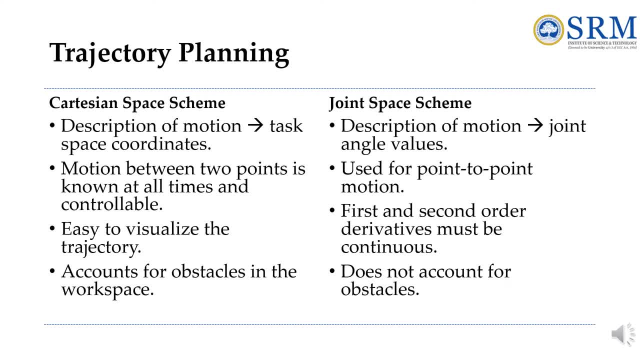 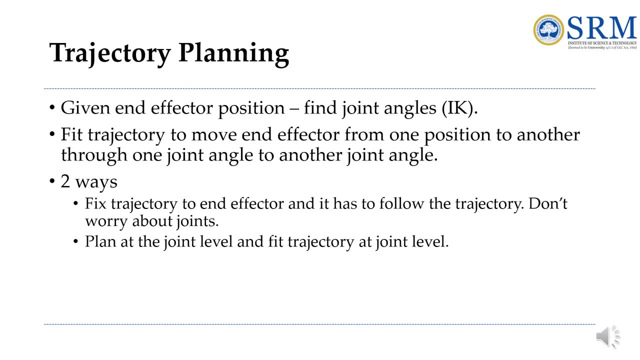 Or by teaching, by showing technique and non-linear nature of manipulator's kinematic model in case of joint space scheme. Then how the trajectory planning is done. given the end effector position, you have to find the joint angles. so first fit the trajectory to move end effector from one position to 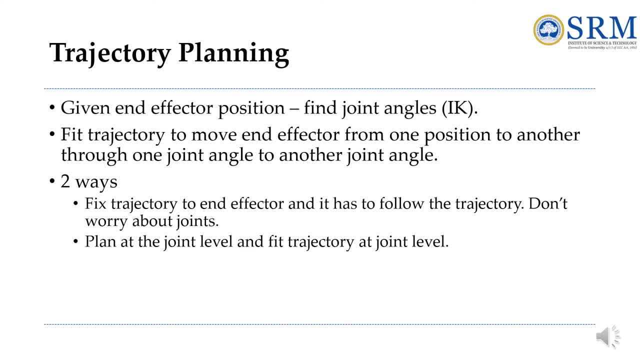 another. To one joint angle, to another joint angle. this can be done by two ways. First, fix the trajectory to end effector and it has to follow the trajectory. The second one is to plan at the joint angle level, that is, and fit the trajectory at that. 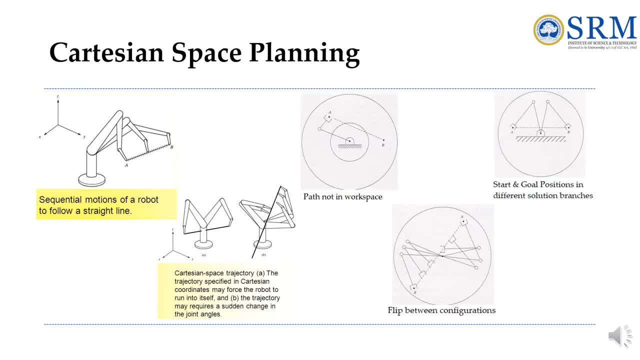 joint level. These picture represents the Cartesian space trajectory planning. the first one shows the sequential motions of a robot to follow a straight line. In the second picture Shows the Cartesian coordinates which force the robot to itself and also it requires us change in the joint angles. 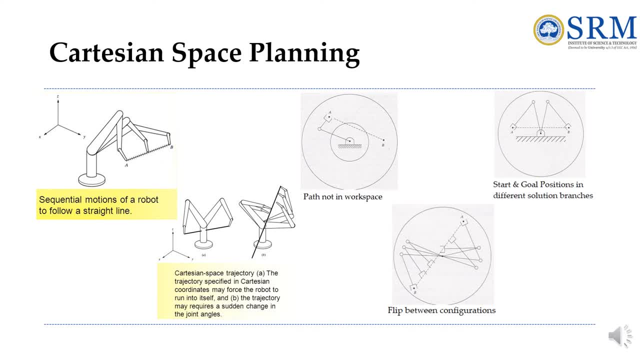 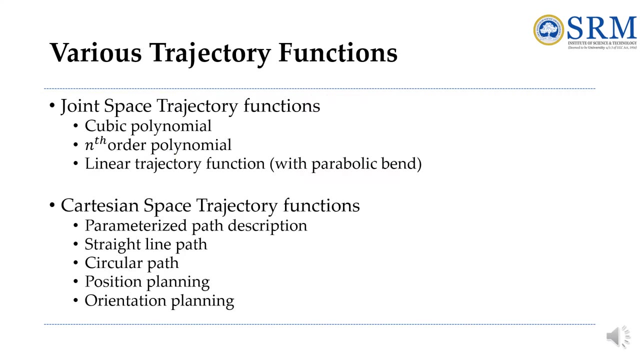 The third picture shows the path which is not in the workspace. In the fourth is it shows the flip between the configurations. and the final one shows the initial and goal positions in different solution branches. So, considering these, we have various trajectory functions And in joint space. 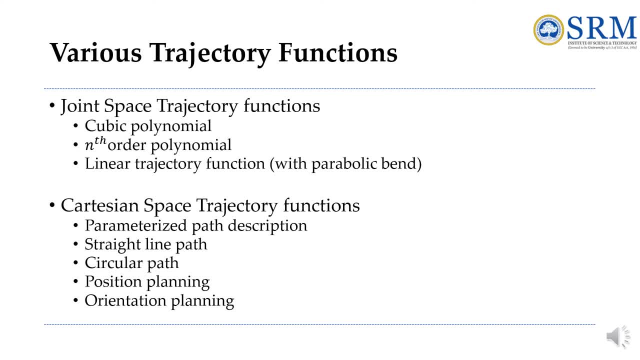 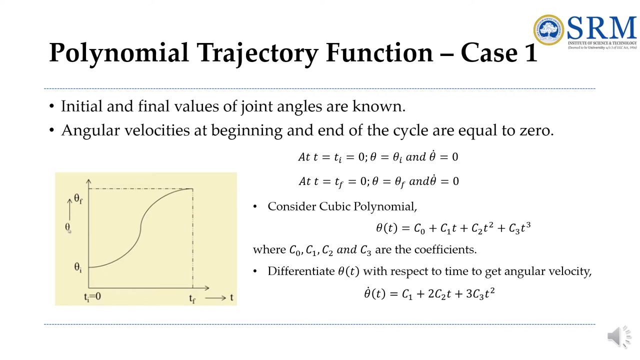 So here initial and final values of joint angles are known, and angular velocities at beginning And end of the cycle are equal to zero. So at t equal to t, i, initial value, which is equal to zero, and theta equal to theta i And theta dot, which is equal to zero. 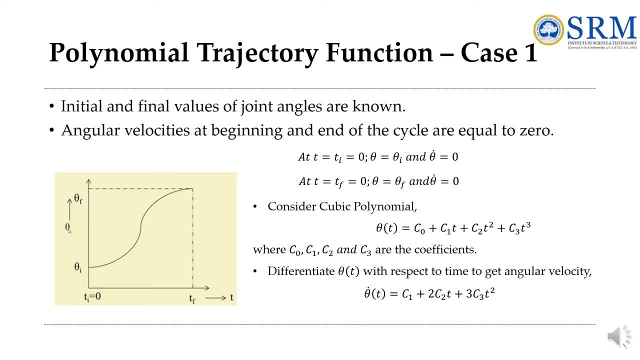 At t equal to t f, the final value is also considered to be zero and theta equal to theta f and theta dot will be equal to zero. Now let us consider the cubic polynomial: theta of t, which is equal to c naught plus c 1 t. 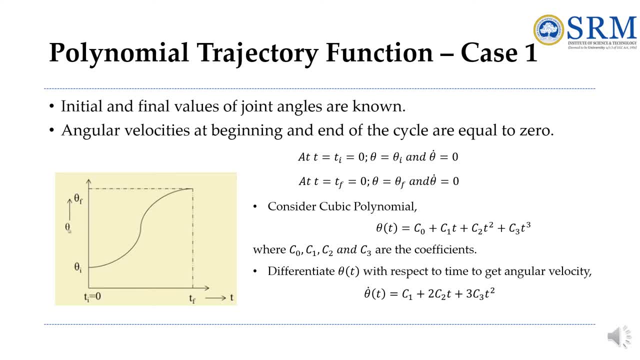 plus c 2, t, Where the c naught c 1, c 2, c 3 are the coefficients. Now differentiate theta of t with respect to time to get angular velocity, So you will get theta dot of t, which is equal to the constant, will be zero and c 1 plus 2. 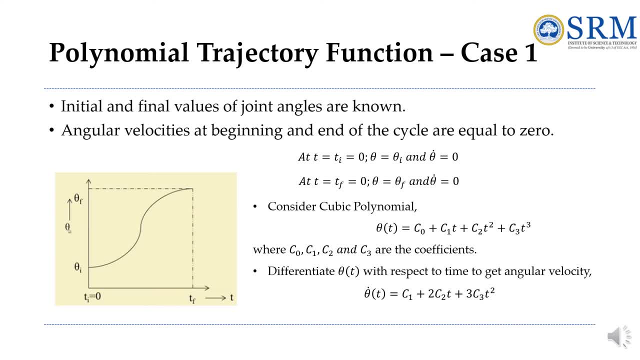 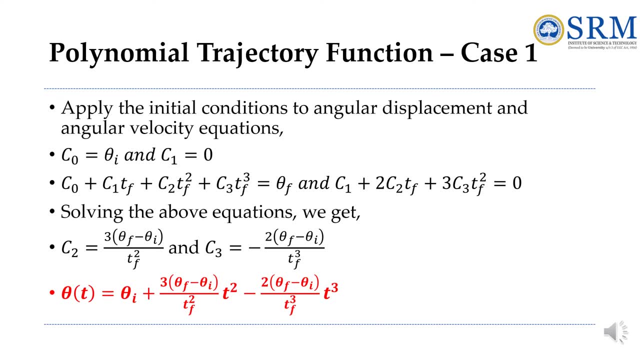 c 2 t plus 3 c 3 t square. Now, applying the initial conditions to angular displacement And angular velocity equations, we get c naught, which is equal to theta i, and c 1 will be zero. Also, c naught plus c 1 t f plus c 2 t f square plus c 3 t f cube, which is equal to theta f. 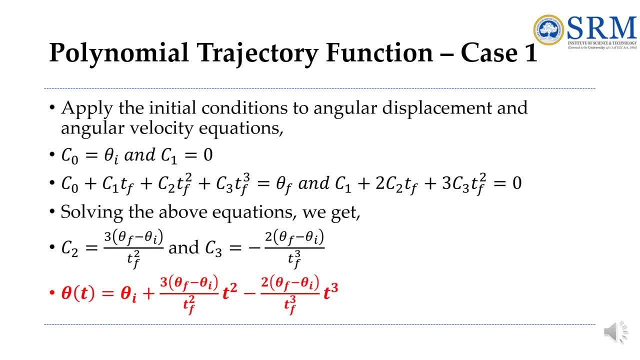 and c 1 plus 2, c 2, t f plus 3, c 3, t f square, which is equal to zero. So, solving the above equations, We get c 2 and c 3 respectively, Where c 2 is equal to 3 of theta f minus theta i by t f square, and c 3 is minus 2 of theta. 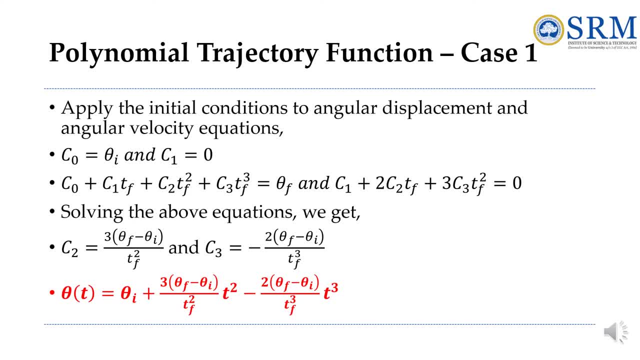 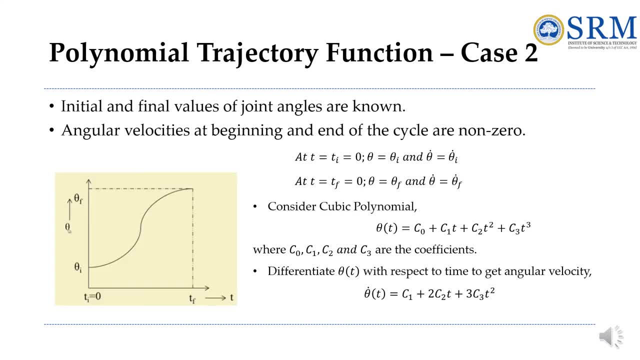 f minus theta i by t, f, cube. And finally, substituting the values of c naught, c 1, c 2, c 3, we get the theta of t. Now consider the case Where c 2. Where initial and final values of joint angles are known and the angular velocities at beginning and end of the cycle are nonzero. here 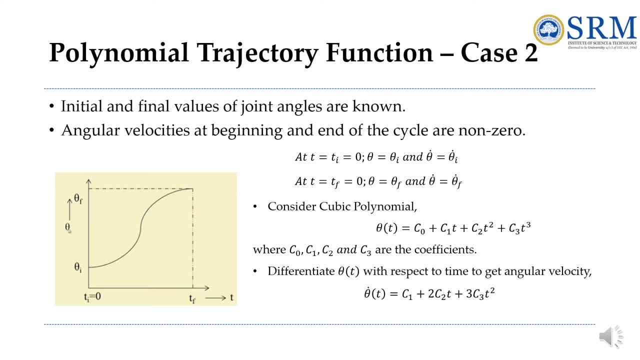 So, which means previously theta, theta dot, which is equal to zero, And here, at initial value, theta dot will be theta i, theta dot i and theta dot, for the final value will be theta dot f. Again, consider the same cubic polynomial And if you differentiate, 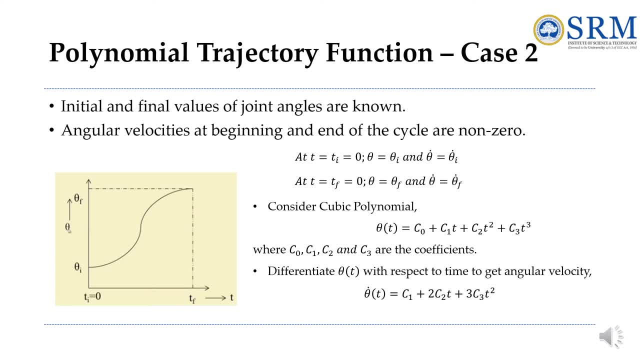 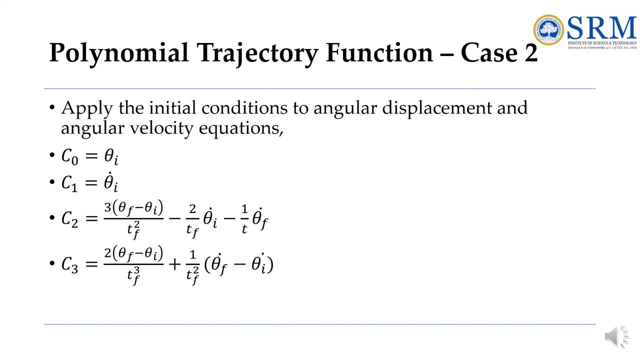 with respect to theta of t, we will get the theta dot of t, which is same as that of your previous equations now applying the initial conditions to angular displacement and angular velocity. equations c naught will be theta i and c1 will be theta dot i- previously it was 0- and c2 and c3 varies. 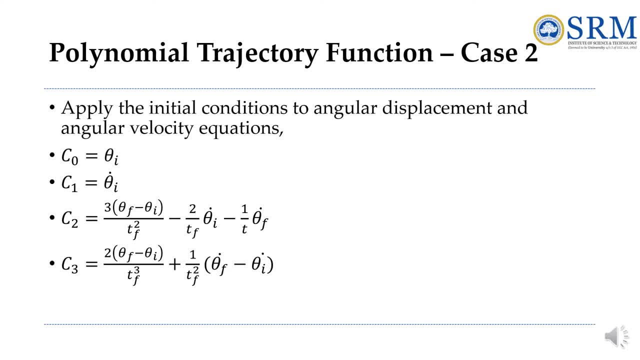 so c2 will be 3 of theta f minus theta i by tf square, minus 2 by tf into theta dot i minus 1 by t theta dot f and c3 will be 2 of theta f minus theta i by tf cube plus 1 by tf square. 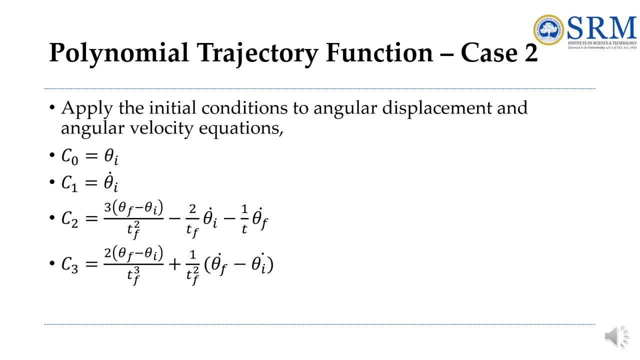 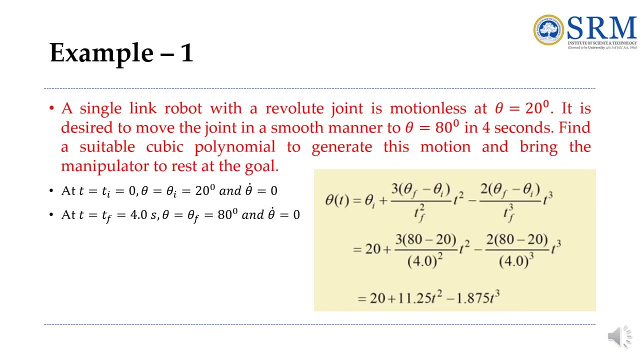 into theta dot f minus theta dot i, so you can assume cases based on the polynomial trajectory function to compute the trajectory path. now let us take this example: a single link robot with a revolute joint is motionless at theta s 20 degree. it is desired to move the joint in a smooth 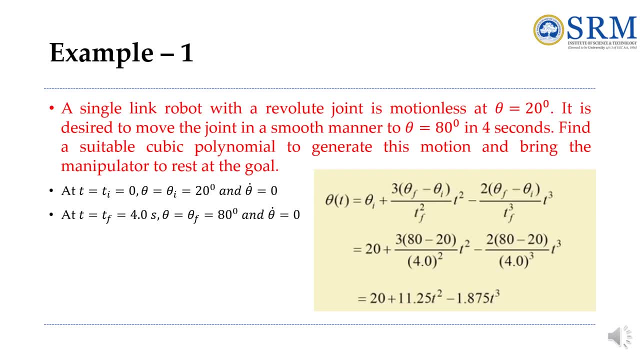 manner to theta s 80 degree in 4 seconds. find a suitable cubic polynomial to generate this motion and bring the manipulator to rest at the goal. so this is your case 1, where initial and final values of joint angles are given and angular velocities at beginning and end of the cycle are. here, it is equal to 0. 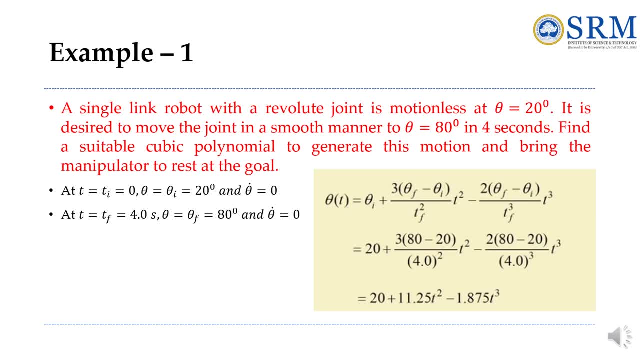 so your initial value is 20 degree and your final value is 80 degree, and the time is given as 4 seconds. so here you will be considering at t is TI, which is equal to 0, and theta is theta, which is 20 degree is given and theta dot. 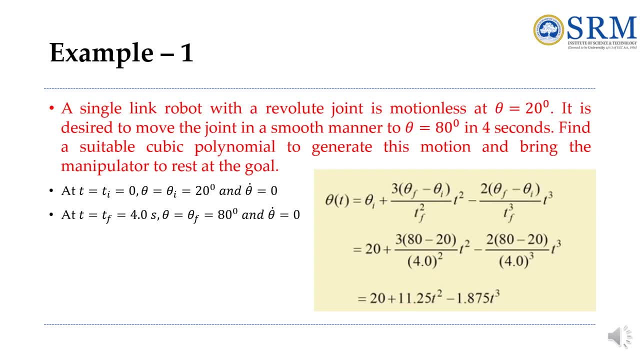 will be 0 and at t is is equal to tf, the time is 4 seconds and theta is theta f, that is, your destination is 80 degree and theta dot. here it will be 0. So this is your case 1.. So, applying the cubic polynomial theta of 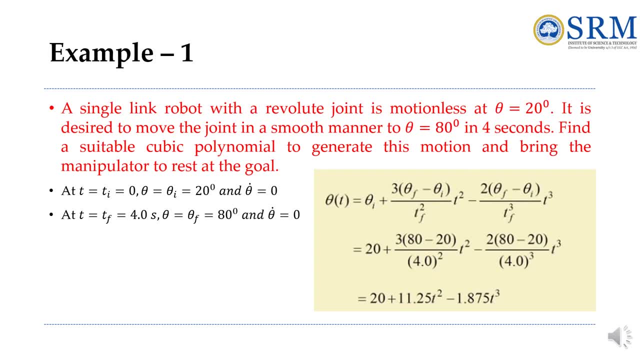 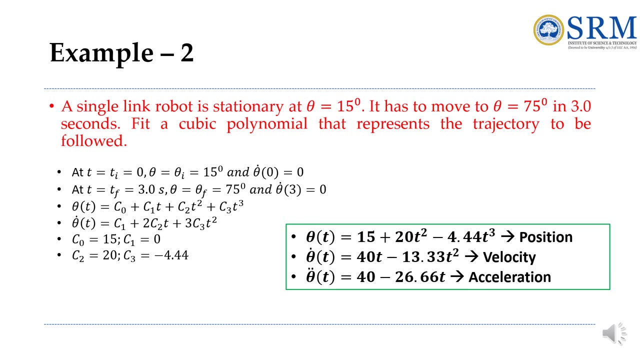 t and substituting the values, you will get the cubic polynomial which will generate the motion and which is bringing the manipulator to rest at the goal. Next, consider another example. a single link robot is stationary at theta is 15. it has to move to. theta is equal to 75 degree in. 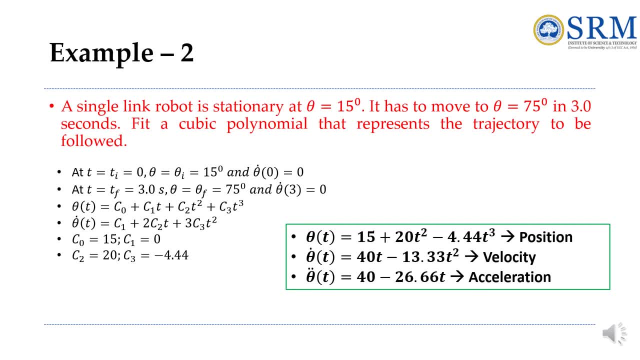 3 seconds Fit a cubic polynomial that represents the trajectory to be followed Here. considering the another way, planning at the joint level- then trajectory has to be fit at the joint level. So, having this, we will be finding the coefficients c, naught, c1, c2, c3 and substitute in theta of t to.